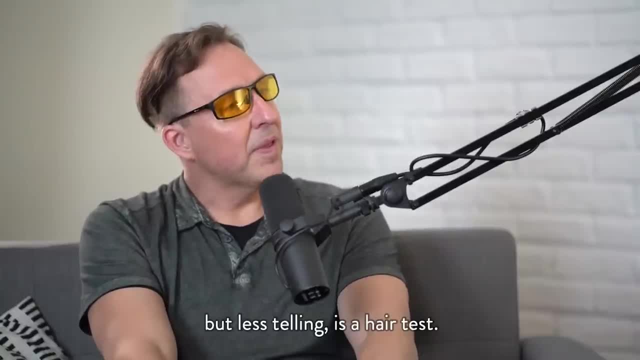 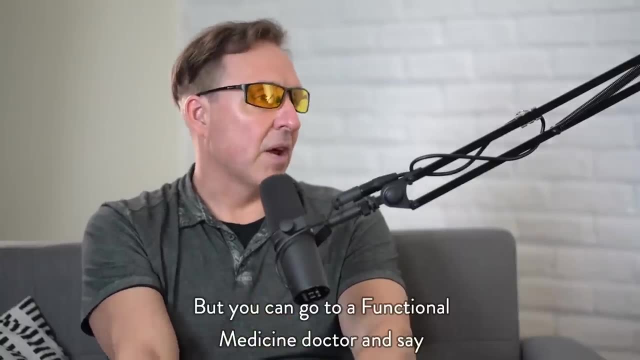 cause you to release more, And then a more common and cheaper way- but less telling- is a hair test, And there's Usefulness for both of those. But you can go to a functional medicine doctor and say I'd like to do a heavy metals test, And they'll usually order a urine test for you. 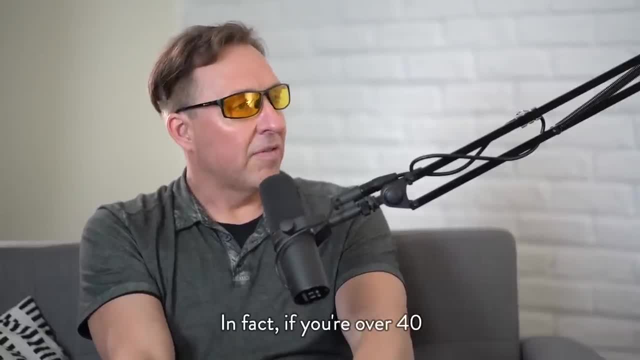 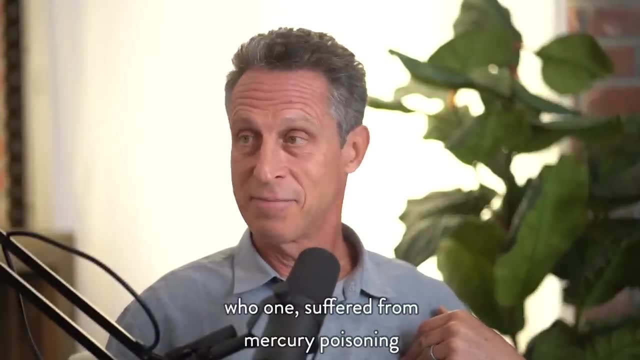 And it's very common to find elevated mercury in lead. In fact, if you're over 40, you're probably going to find it. Yeah, So here let me just share with you, as a practicing physician, who one suffered from. 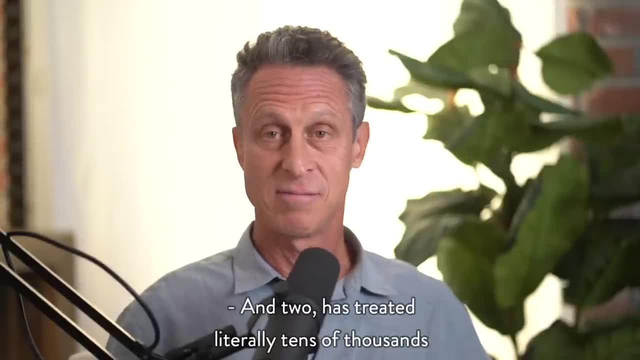 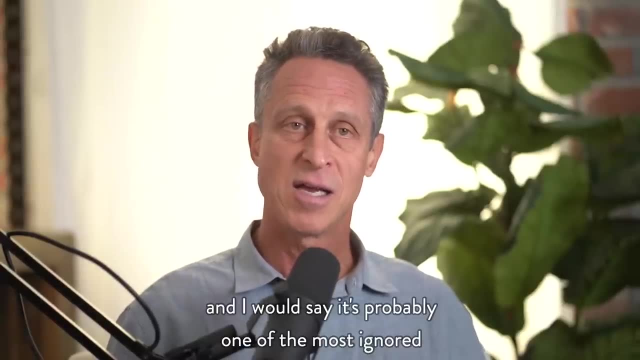 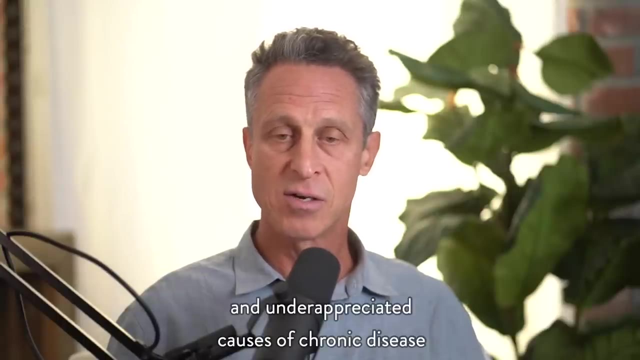 mercury poisoning Added two And two have treated literally tens of thousands of people with metal poisoning and have done tens of thousands of tests, And I would say it's probably one of the most ignored and underappreciated causes of chronic disease that doctors don't know how. 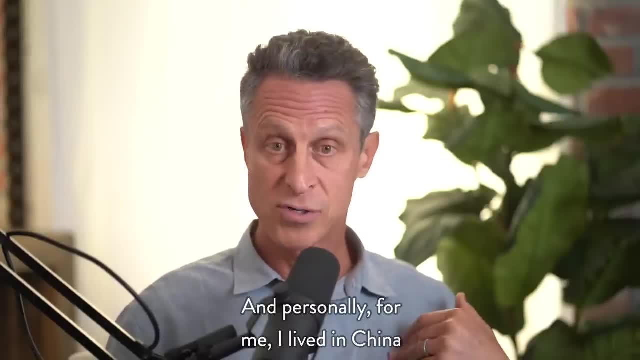 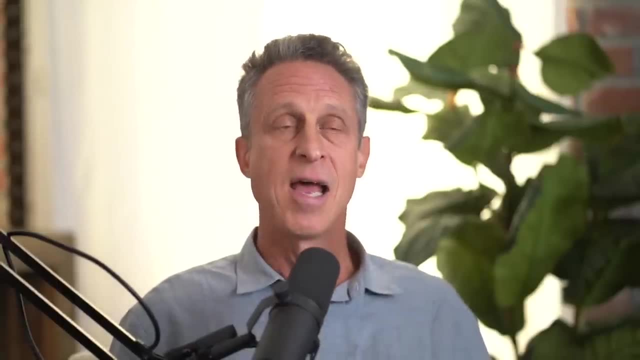 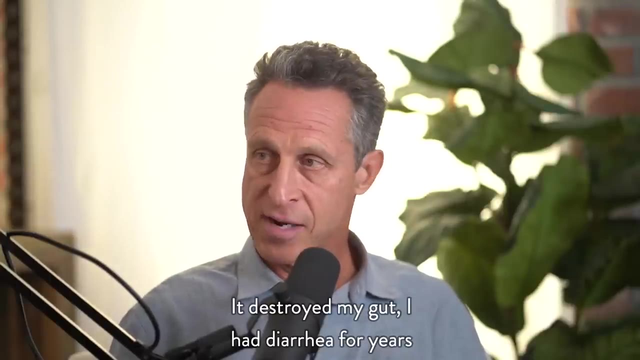 to think about test or measure And personally for me. I lived in China and it got huge exposure to mercury- I don't have great genes at detoxifying And it destroyed every system in my body. It destroyed my gut- I had diarrhea for years and bloating and pain. It destroyed my 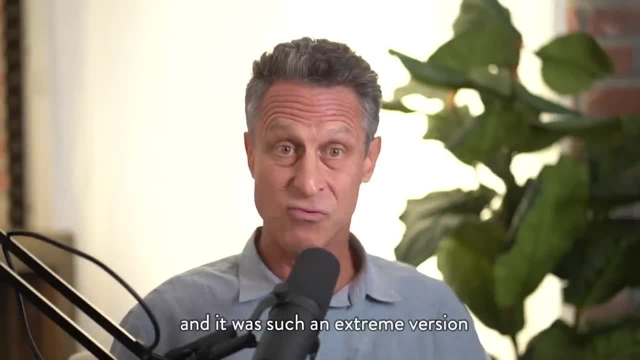 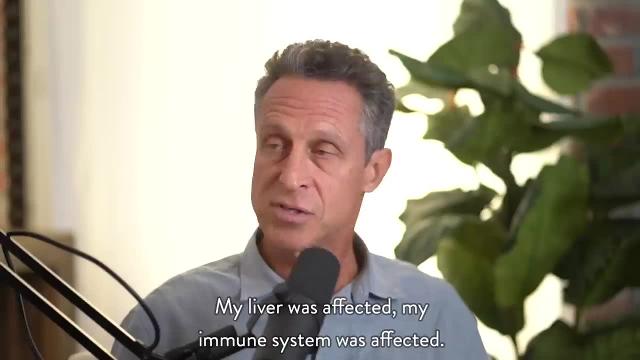 mitochondria. I developed chronic fatigue syndrome And it was such an extreme version that my muscle enzymes were high. My CPKs were like 600.. My liver was affected. My immune system was affected. I started developing rashes and sores all over. I was completely cognitively. 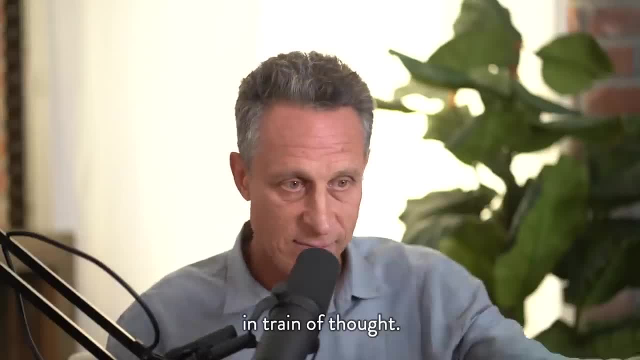 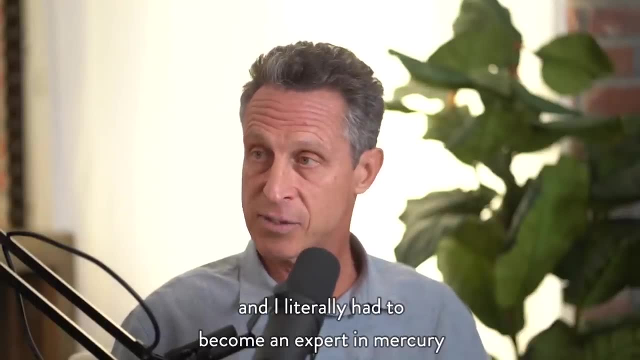 impaired, I couldn't focus, think, concentrate. remember where I was, you know, in train of thought, You're not in a good place. Yeah, This was, like you know, 25 years ago And I was so bad And I literally had to become an expert. 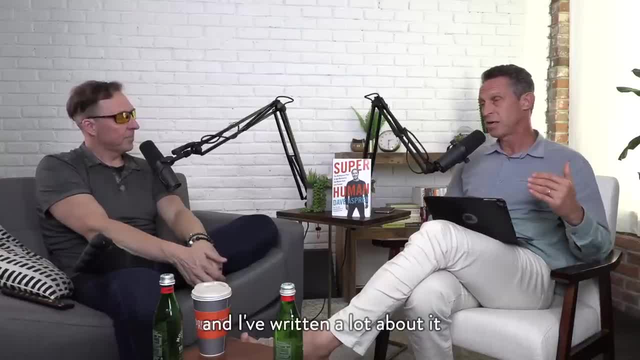 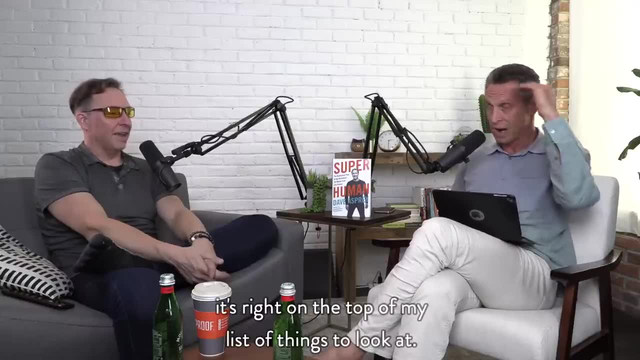 in mercury and heavy metals and detoxification And I've written a lot about it, But I think you know I would say that for many of my patients who suffer from weird or strange ailments, it's right at the top of my list of things to look at. 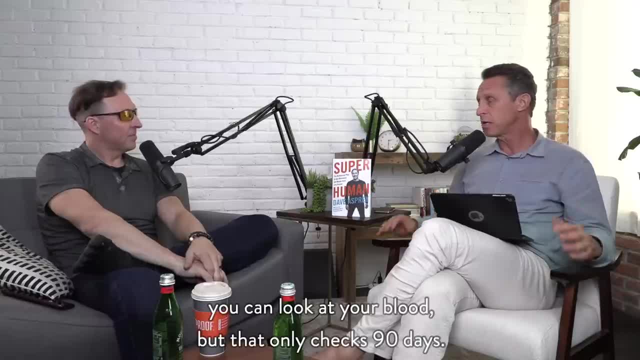 And the only way to really know what your body burden is. you can look at your blood, but that only checks 90 days. I mean, if you're eating a lot of sushi you'll see it's high, But 90 days. 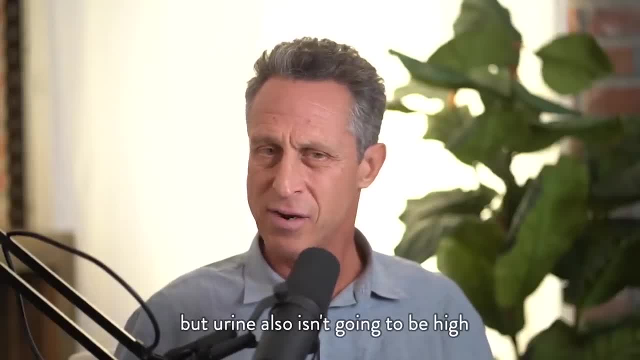 you stop, it'll go away. You can look at your urine, but your urine also isn't going to be high unless there's an occurring exposure. So if you're in a lead foundry or you're, you know, eating tons of sushi, you might see a lot of blood. But if you're in a lead foundry or you're, you know, eating. 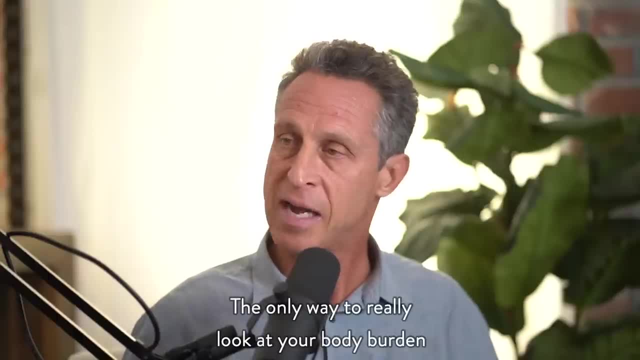 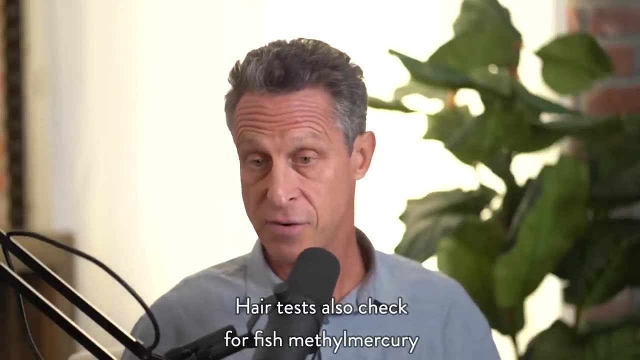 tons of sushi, you might see a little bit of mercury. The only way to really look at your body burden is to do a challenge test where you take a pill- it's a chelator- and you collect your urine for six hours. Hair tests also check for fish methylmercury, which is where we mostly get. 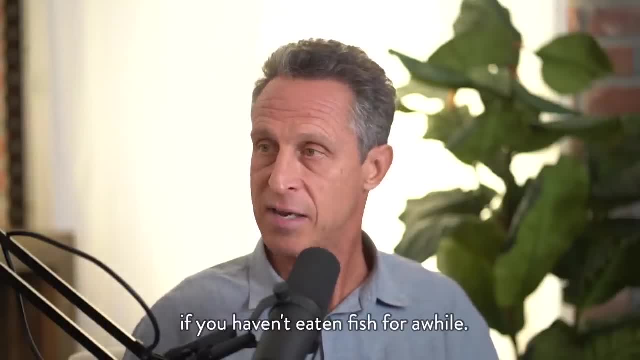 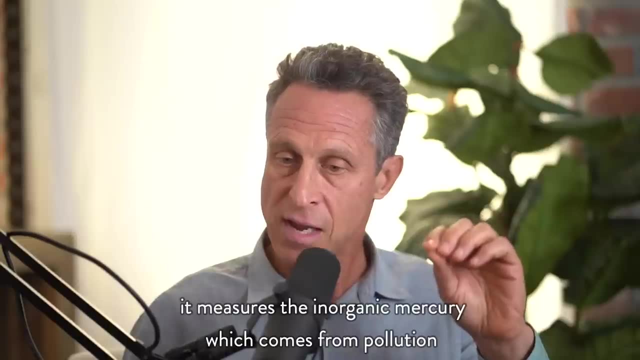 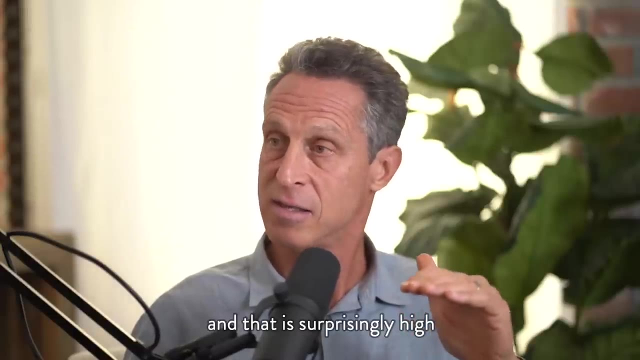 our mercury from, But that also will go away if you haven't eaten fish for a while. And then there's another test that looks at the blood work, that measures the inorganic mercury which comes from pollution or from fillings, And that's called the Quicksilver test And that is surprisingly high in people who have a mouthful. 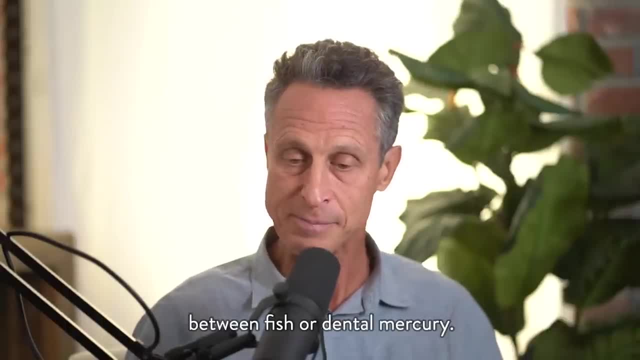 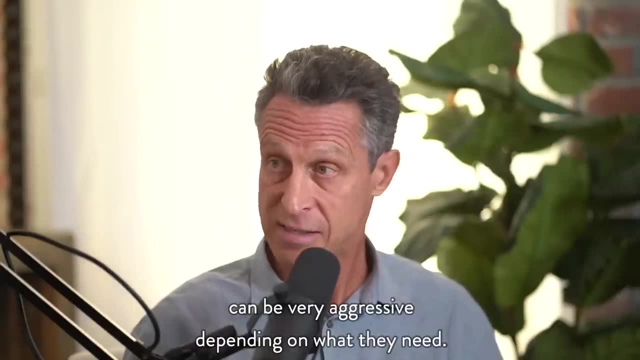 of fillings And you can see the difference between fish or a dental mercury And the treatments are depending on the person. you know can be very aggressive depending on what they need. I have a patient who's got this terrible autoimmune disease and we're giving her 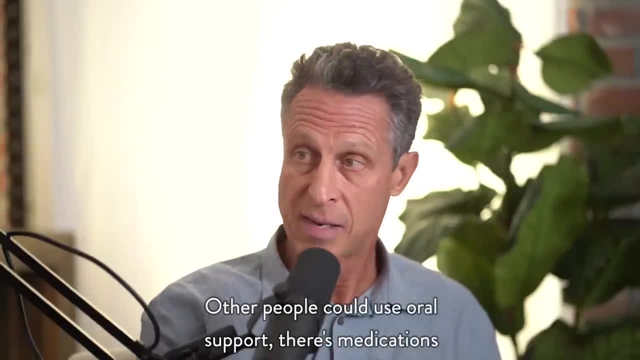 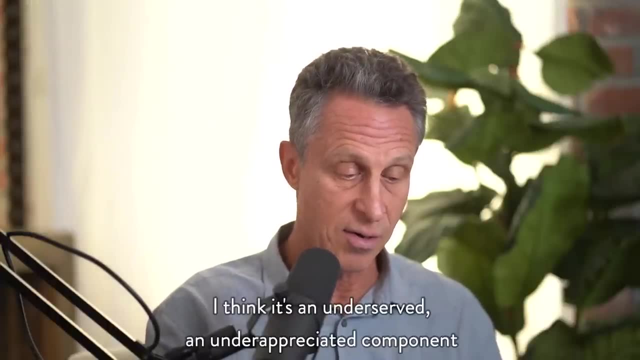 intravenous support. Other people can use oral support. There's medications, But it's a whole process that has to be done safely And I think your point is really well taken. I think it's, you know, an under-served, an under-appreciated component of medicine And hopefully one day we'll 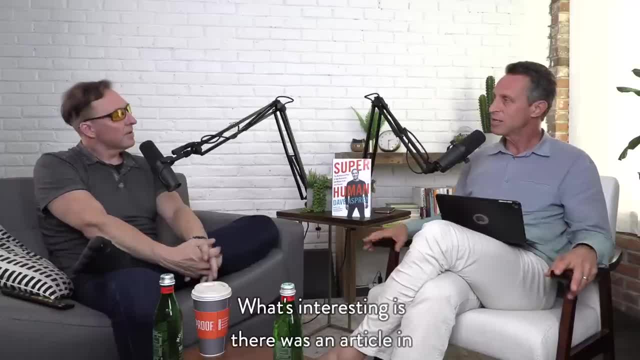 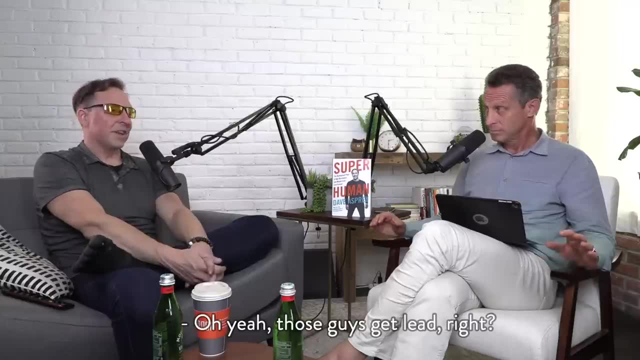 get on board with this, because it's just. I mean, it was interesting. There was an article in the New York Times that I was quoted in. It was based on these special forces. Oh yeah, Those guys get led right. 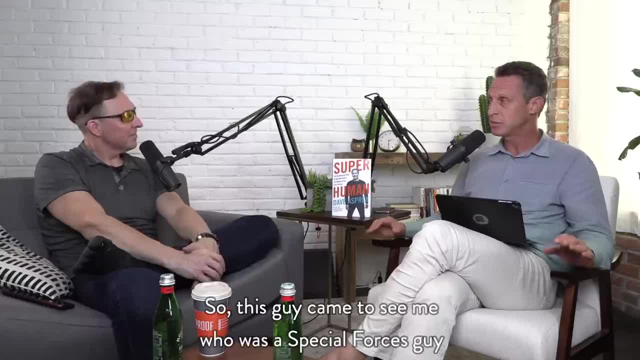 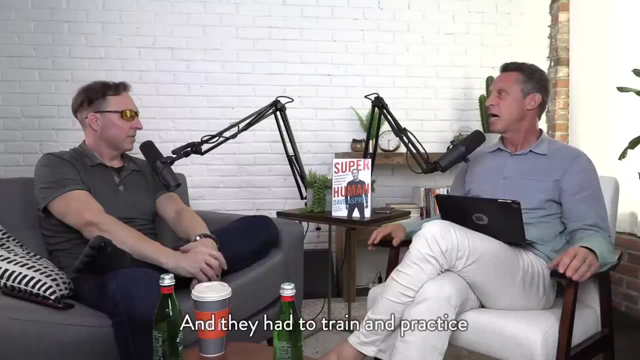 Yeah, So this guy, this guy came to see me whose job was? he was a special forces guy who was a blast expert, So they would, you know, go blow up stuff, you know, blow up doors, blow up this. And they had to train and practice. 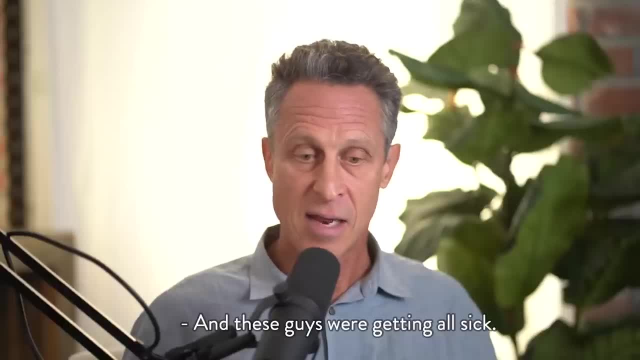 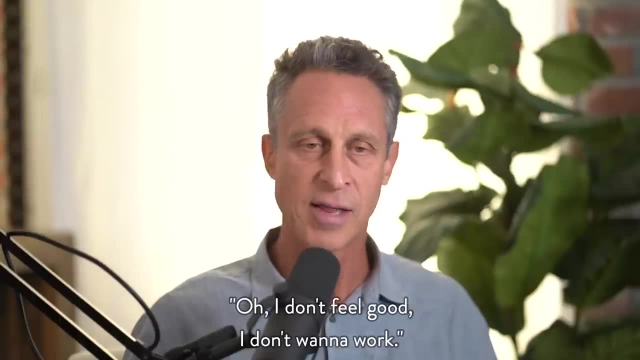 And they had indoor practice training And these guys were getting all sick. And now you know, the special forces guys aren't malingerers, They're not whiners, They're not like, oh, I don't feel good, I don't want to work. Those aren't those guys. These are the guys. 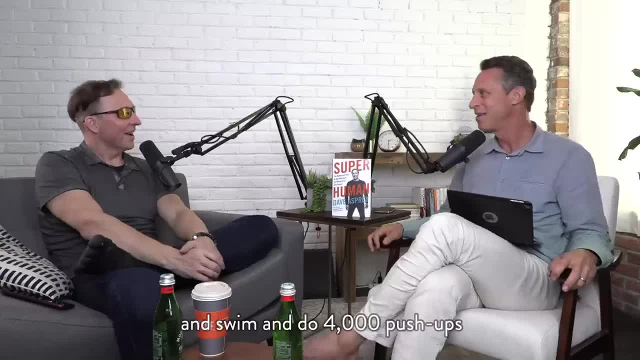 who you know like stay in freezing ice water for an hour and swim, you know, and do 4,000 push-ups and, like you know, don't sleep for three days. I mean, these guys are not whiners. 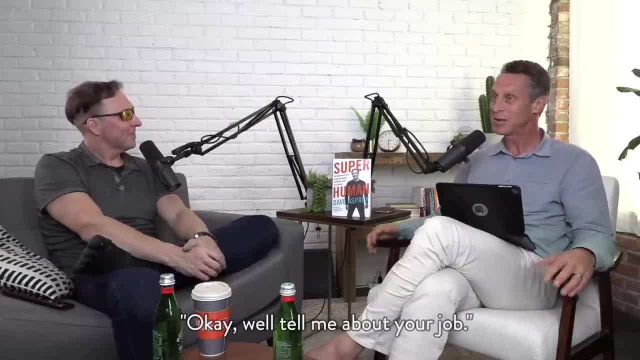 They're superhumans, right, Yeah? And so the guy came in. I'm like: okay, well, tell me about your job. I'm like, oh, we blow stuff up, We shoot things. I'm like, oh, okay. And so I said, let's check your heavy. 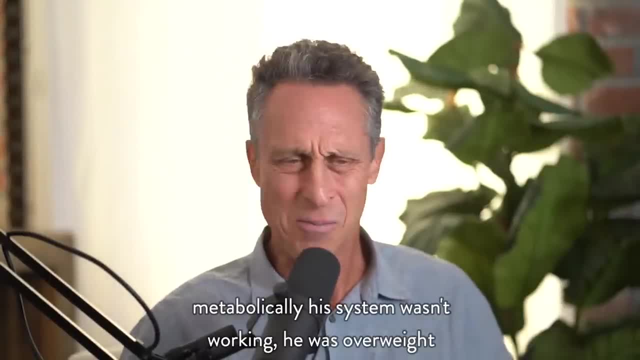 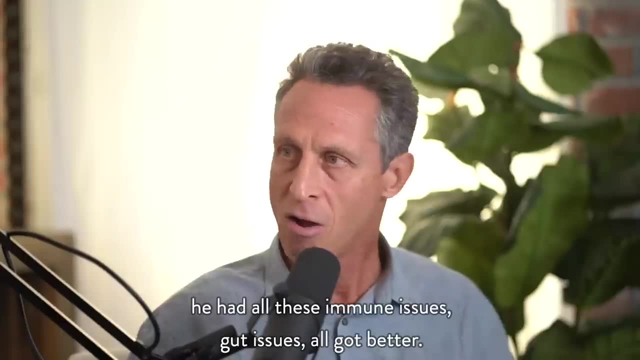 metals And they were sky high. We put him through a whole program. He was, you know, metabolically, his system wasn't working. He was overweight, He had prediabetes, He had cognitive dysfunction, He had all these immune issues, gut issues. All got better And then he started sending all these special forces guys to us And we started treating them And they just all got better. And one of them was written about in the New York Times: Wow, Because his- you know- medical crew and everybody dismissed him And he completely turned around. 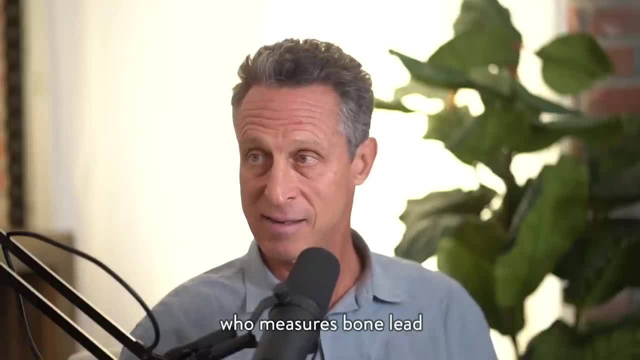 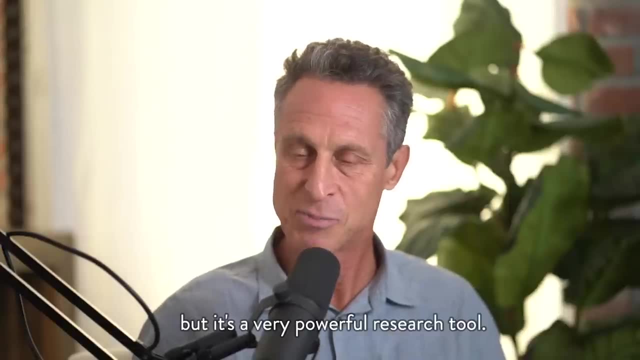 The guy who is the lead expert at Mount Sinai who measures bone lead, which is the most accurate way to measure lead in the body. It's not an easy, available commercial test but it's a very powerful research tool. He said these guys had really high levels of lead. 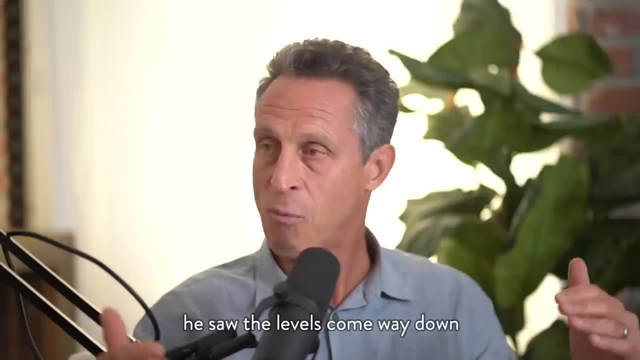 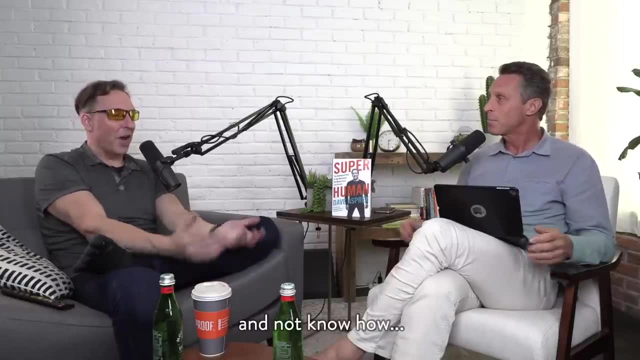 And he said on the follow-up test he saw the levels come way down. And he says he's never seen that in his entire experience. And this is a guy who's an expert in lead. How can you be an expert in lead and not know how to blow the body? It drives me nuts. Because it's not seen as a problem. Acute poisoning, yes. Chronic poisoning, no. And there's nothing you can quote do about it. It's just nonsense. And there's in fact an FDA-approved drug called DMSA. It's designed for lead removal and actually removes mercury. 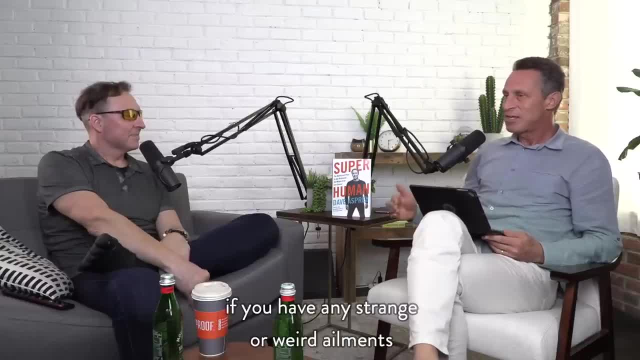 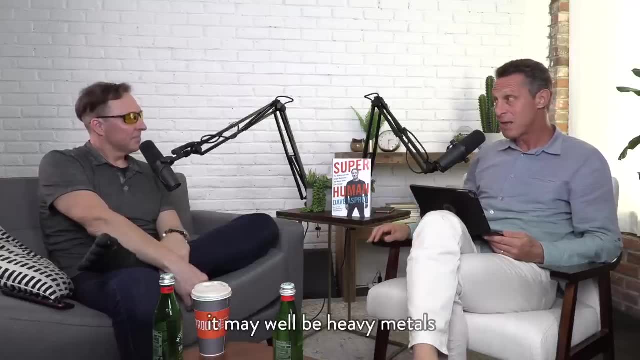 So I think you know, for people listening, if you have any strange or weird ailments. if you have anxiety, depression, insomnia, autoimmune disease, gut issues, fatigue, cognitive issues- it may well be heavy metals And you need to find a good functional medicine. 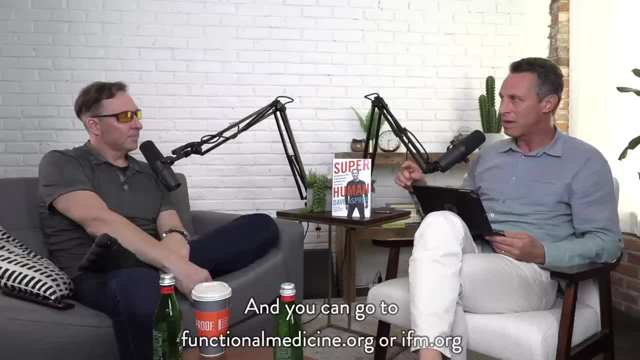 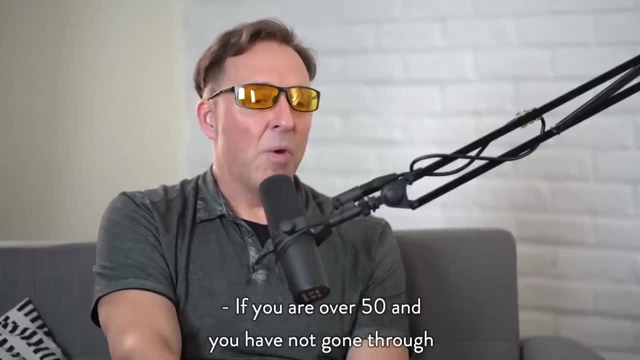 doctor to help you diagnose that And you go to functionalmedicinecom Or ifmorg And you can find a practitioner who may know how to do this. I'm going to go a little bit broader than that. If you are over 50 and you have not gone through, 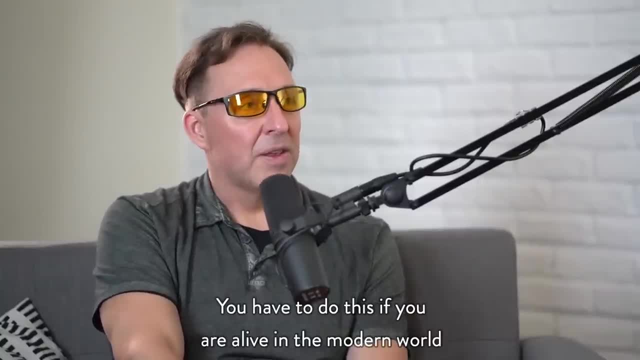 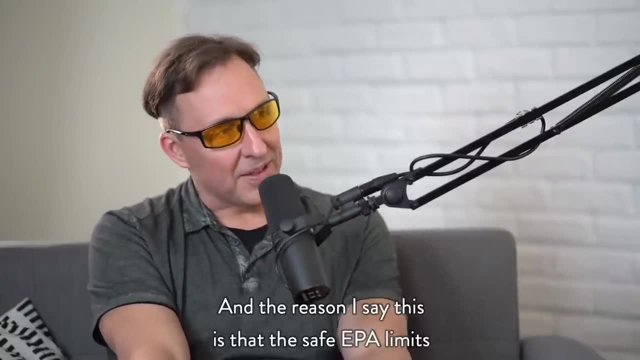 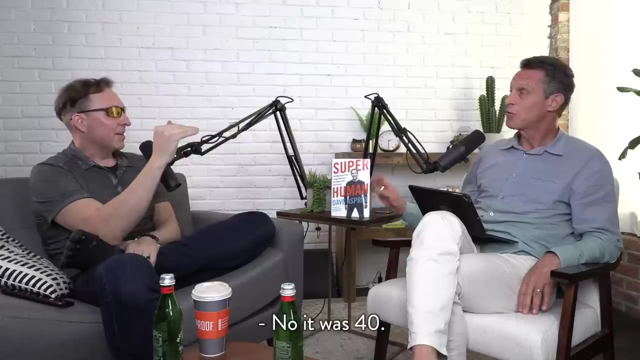 a course of chelation. you are not doing aging right. You have to do this if you are alive in the modern world and you want to live to a highly functional old age. And the reason I say this is that the safe EPA limits for lead used to be 20 parts per million, And they cut it. 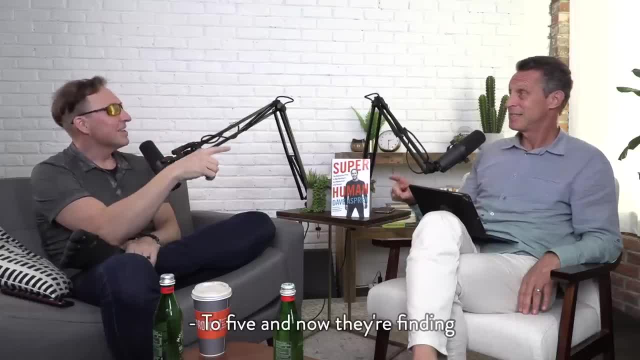 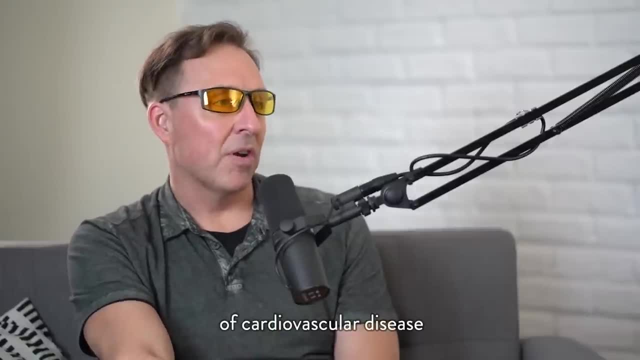 It was 40. It was 40. It was 20 to 10 to 5. 5. And now they're finding even down to 1, they're seeing cognitive impairment in kids, Cognitive impairment and increased risk of cardiovascular disease. And now the people. 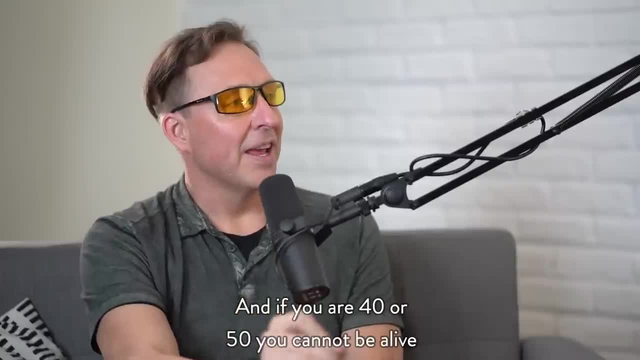 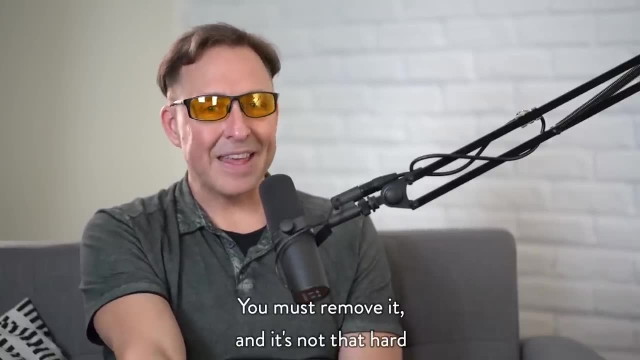 who are the experts in lead are saying: quote: there is no safe limit of lead And if you are 40 or 50, you cannot be alive and not have a lead burden in your body. You must remove it, And it's not that hard, especially if you're not really sick, It's not going to be a big deal. 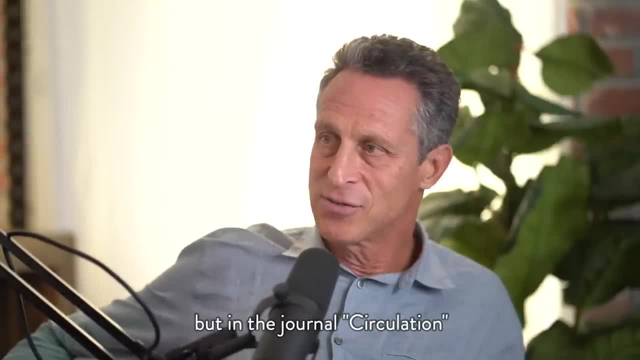 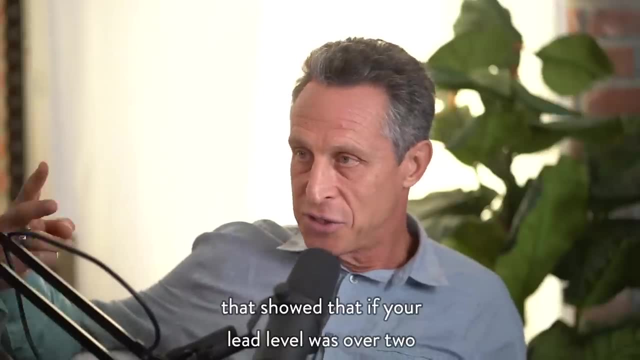 And it's so strange, Dave, because medicine just ignores this, But in the journal Circulation, which is one of the Top cardiology journals, there was a paper a number of years ago that showed that if your lead level was over 2, which is, quote, within the normal limits, which, by the way, affects 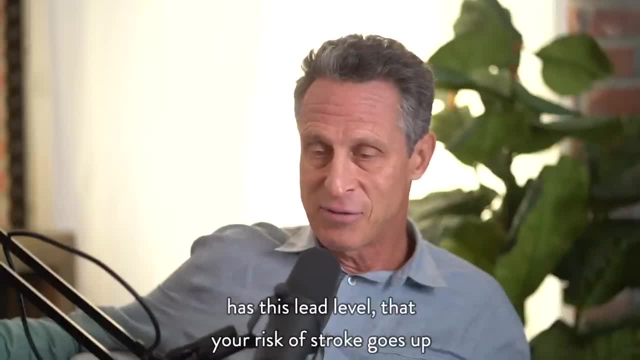 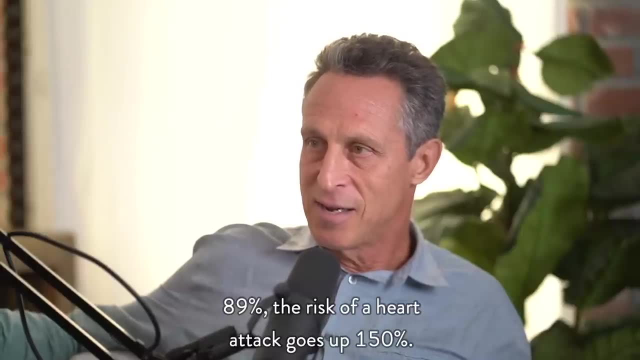 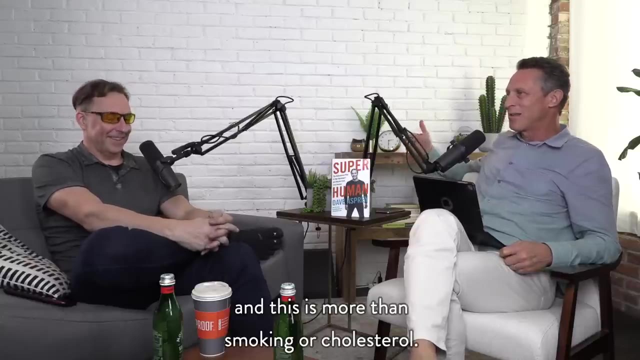 almost 40% of the population has this lead level- that your risk of stroke goes up 89%, The risk of a heart attack goes up 150%. The risk of death goes up from a heart attack 55%, And this is more than smoking or cholesterol. 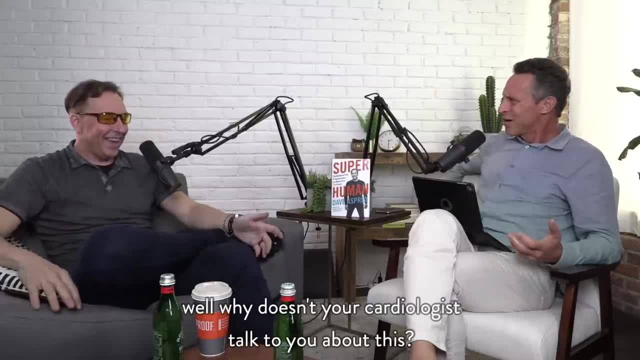 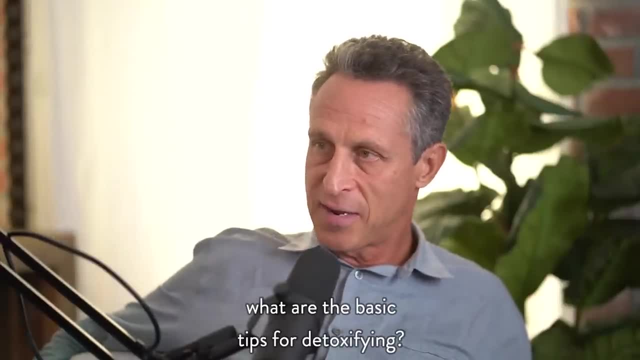 Oh, and it's like: well, why doesn't your cardiologist talk to you about this? So what are the basic tips, if you're not going to get chelated? What are the basic tips for detoxifying? For detoxifying not just metals, Or you mean metals. 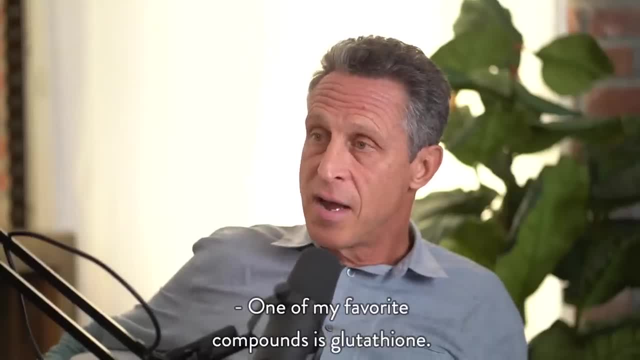 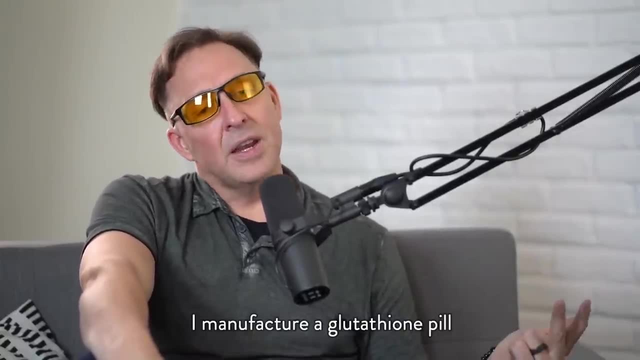 No metals. It all works for everything, But how do you? One of my favorite compounds is glutathione And you can increase glutathione levels by increasing vitamin C, by taking N-acetylcysteine. I manufacture a glutathione pill You can get. 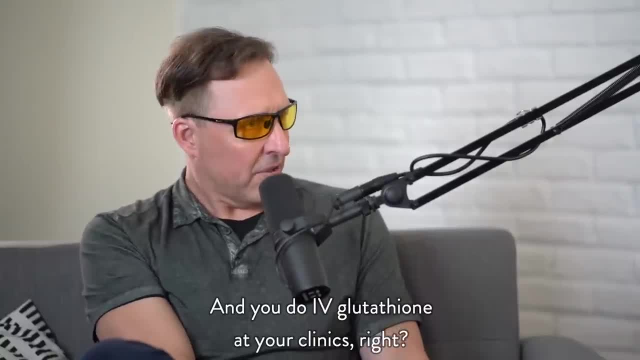 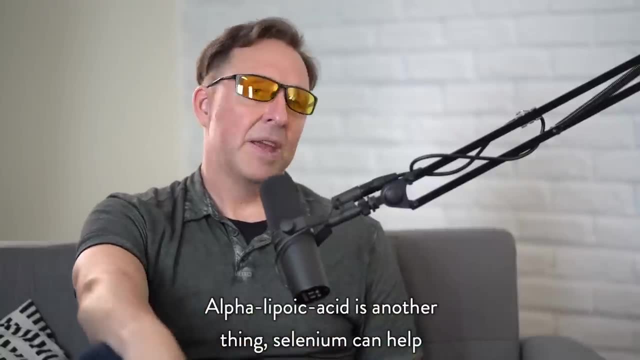 intravenous glutathione, which Like coaxial, Yeah Yeah, And you do IV glutathione at your clinics, right? Yeah Yeah, And we do it at Upgrade Labs in LA for people to recover better. Alpha-lipoic acid is another thing. Selenium can help And 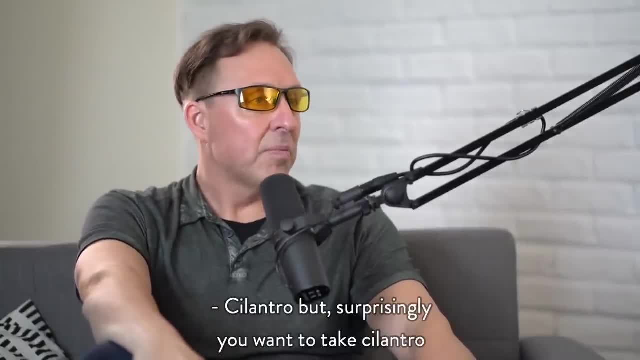 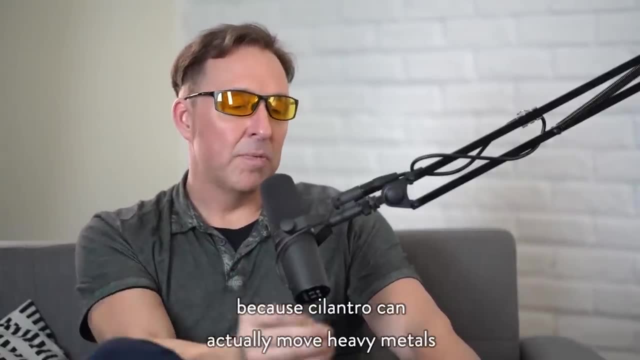 Zinc. Zinc can help The natural chelator, Cilantro, But surprisingly you want to take cilantro only after you've removed most of the metal from your body, because cilantro can actually move heavy metals into the brain, because it's one of the things that can also penetrate the blood barrier. So you go through and you say: you know, I'm just going to build, Yeah, I'm going to build some of these in on a regular basis. And then you need fiber, You need to poop and pee and sweat. Shocking how those work. 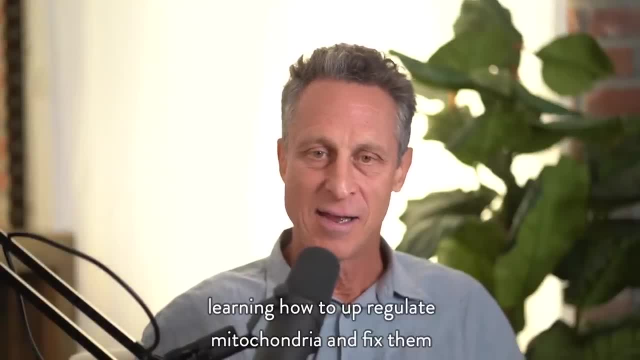 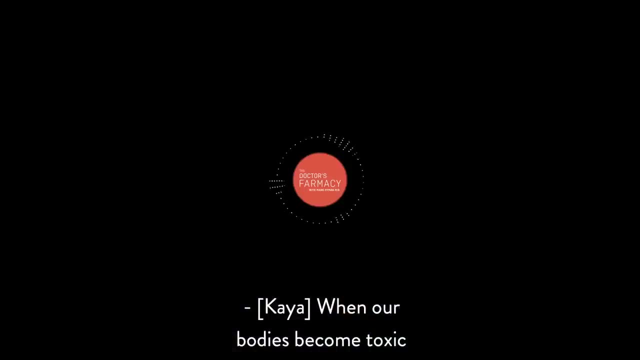 Yeah, Metals are a real deal. And learning how to detoxify, learning how to up regular mitochondria and fix them, learning how to cool off inflammation: These are the central strategies around healthy aging. Yeah, When our bodies become toxic, every one of our systems can become affected. This is just 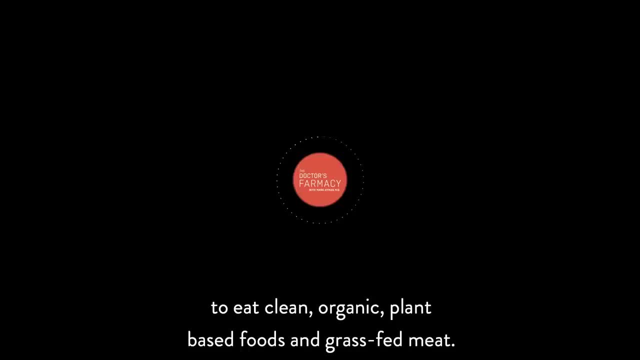 one of the reasons why it's so important to eat clean, organic, plant-based foods and grass-fed meat. Eat plenty of cruciferous veggies like broccoli, bok choy and other vegetables that are good for you. Yeah, You can also enjoy kale and Brussels sprouts to maximize your dietary phytonutrients and